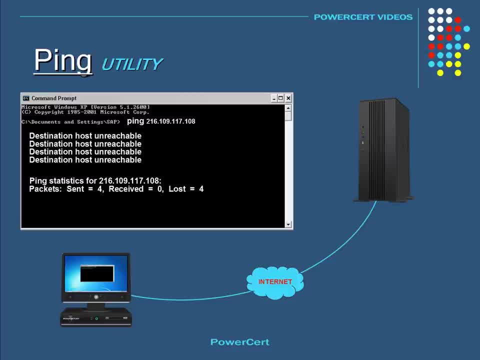 then that message is coming from a router And it means that a route to the destination cannot be found. The ping command can also be used to test name resolution, For example, before we used the ping command with an IP address, But we can also use it with a domain name. 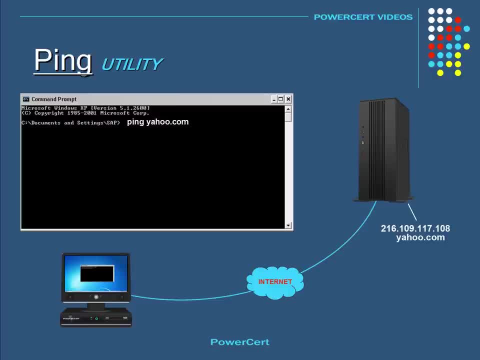 For example, we could type ping space, then the domain name yahoocom. So by pinging the domain name, if we got the same successful result as typing the IP address, then this would indicate that name resolution by DNS is working fine. But let's just suppose that the domain name ping failed. 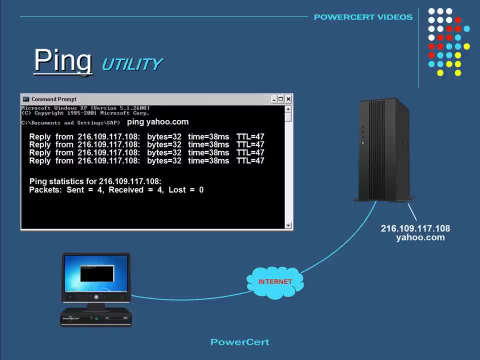 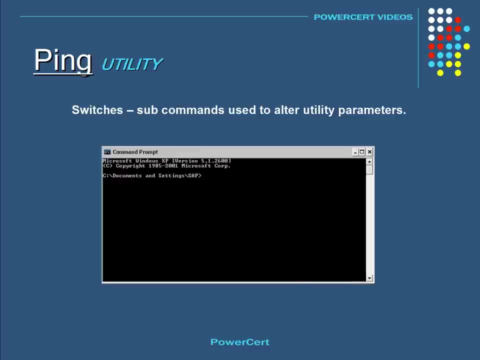 Then the next step would be typing the IP address instead. So if by typing the IP address, if the ping command was successful this time, then we now know that we are having a problem with DNS. The ping command can also be combined with other subcommands called switches. 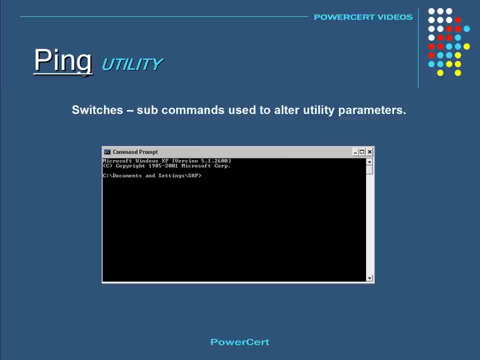 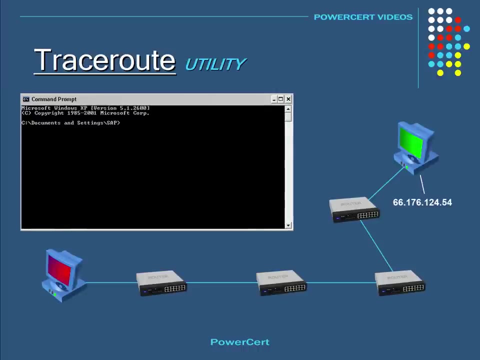 Switches are used to alter the parameters of the ping utility. You can view a full list of these switches by typing ping, space, forward, slash and then a question mark. Our next utility is called traceRT, which stands for trace route. This utility is used to see the IP address. 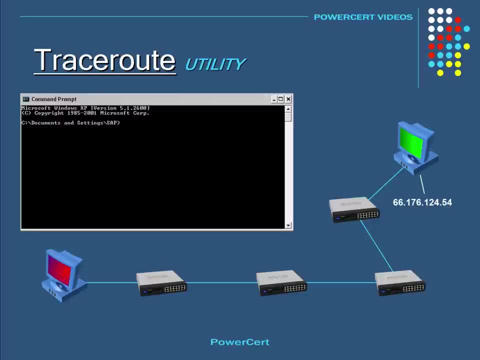 We can see the exact path the data packet is taking on its way to the destination. So for example, let's go ahead and trace the route from our computer to another computer. So at a command prompt we would type traceRT, space and then the IP address and press enter. 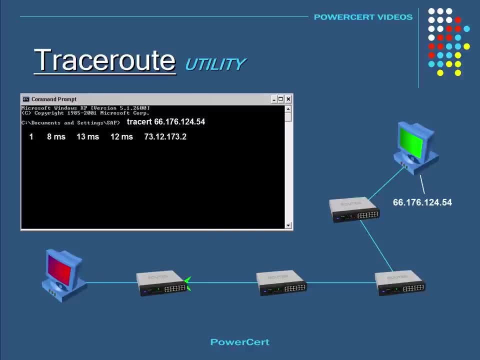 Now the data packet will find its way to the destination, And each time it reaches a router on its path, it will report back information about that router, such as the IP address and the time it took between each hop. So the traceRT utility is a great tool that can be used to pinpoint where a problem lies on a network.